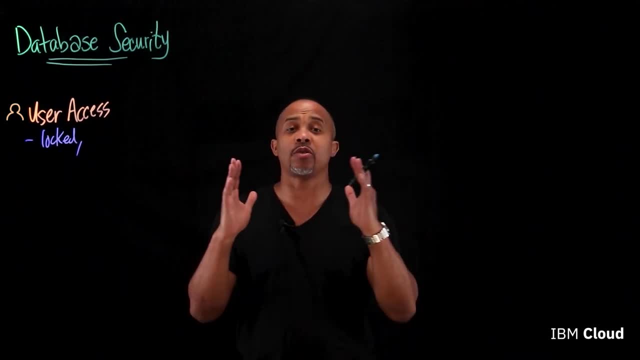 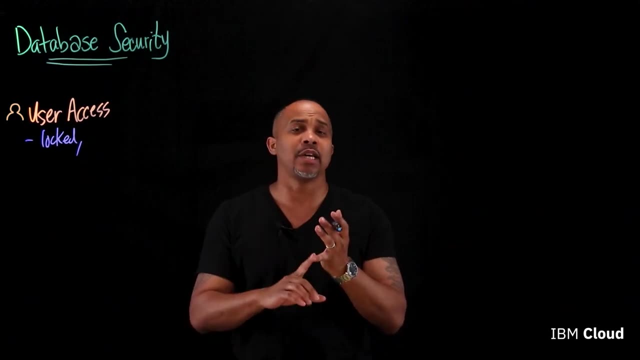 It's very common. It's very useful to, or convenient to, put all of these components on one server, But what does that really expose you to? Let's say you're doing a LAMP stack, Linux, Apache, MySQL, PHP- and there happens to be a compromise. 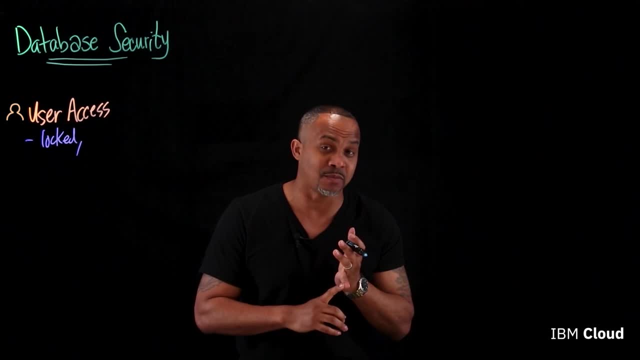 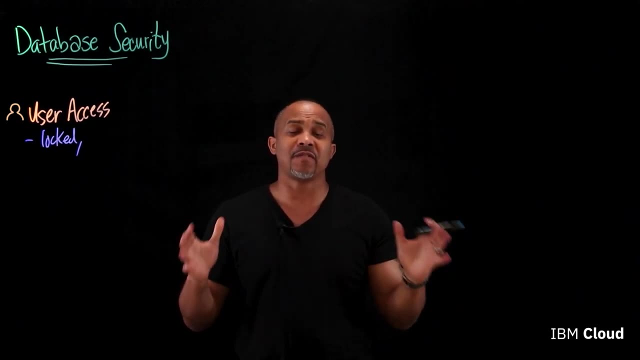 We know from there that there are two things that can be compromised. You have the operating system and maybe something in the PHP code, particularly a vulnerability that could happen here. So in the event that something does get compromised, another best practice to take into consideration. 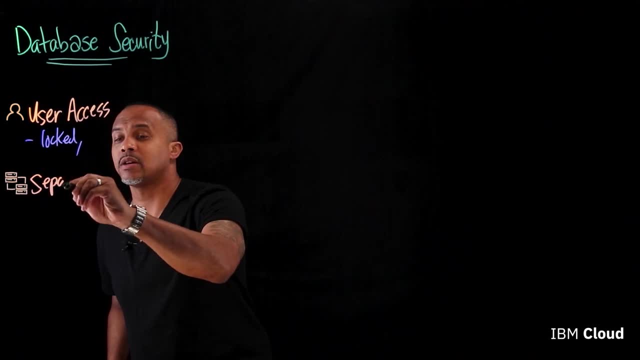 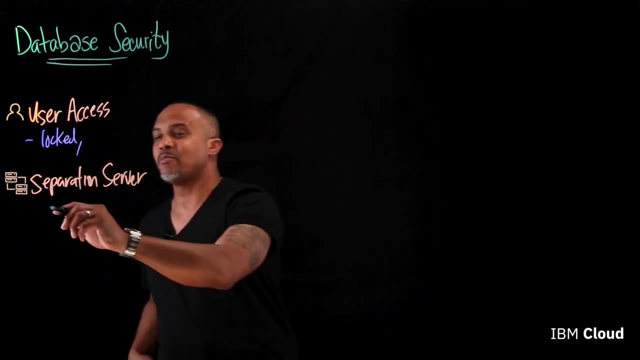 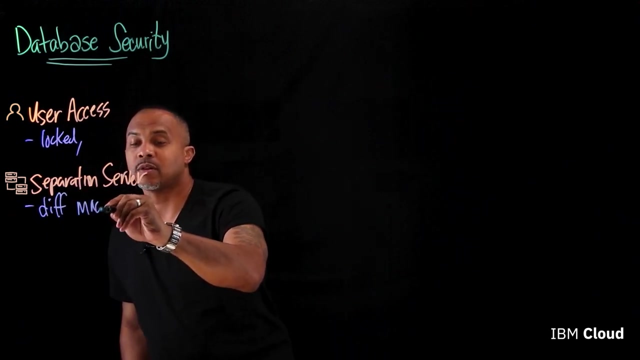 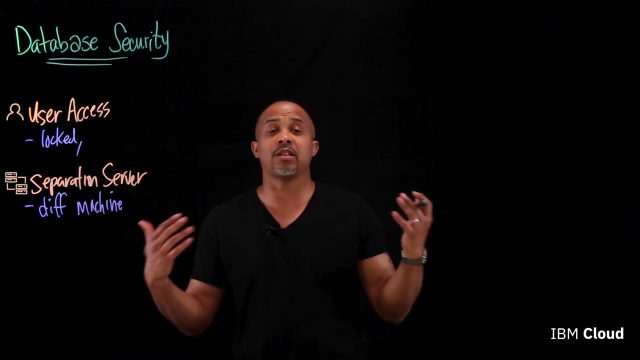 is to have separation, And I'll just say of server here. Do some shorthand code here. So maybe you want to run that on a separate machine. Okay, So it'll be separated. So in the event that something does happen, maybe at a Linux OS level, 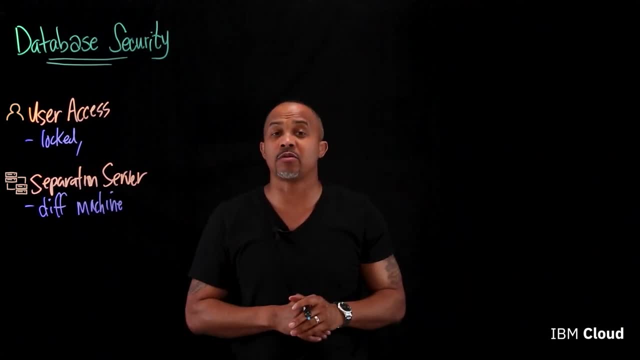 you have the ability that data is set apart, Okay. Okay, So you have another machine that you can really isolate what happens there as well. This is especially important if you have an e-commerce business occurring for you Now, if you are subscribing to a SaaS service that runs your e-commerce application. 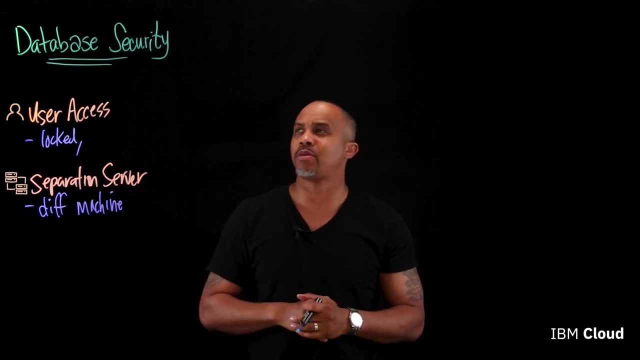 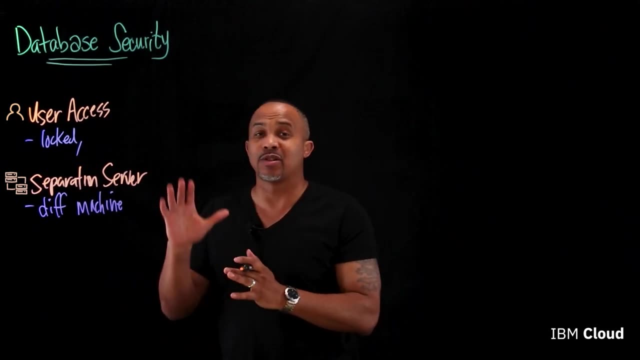 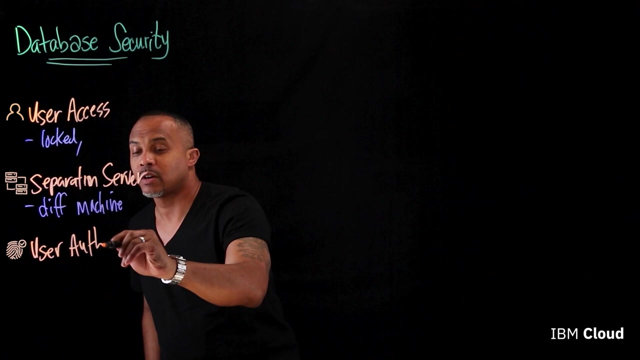 do a little checkout, Ask some questions about: do they have some of these practices in place? Next, let's deal with the actual access to the system. We talked about physical access. Let's talk about user access Now I believe, if I can quote a recent Verizon survey- 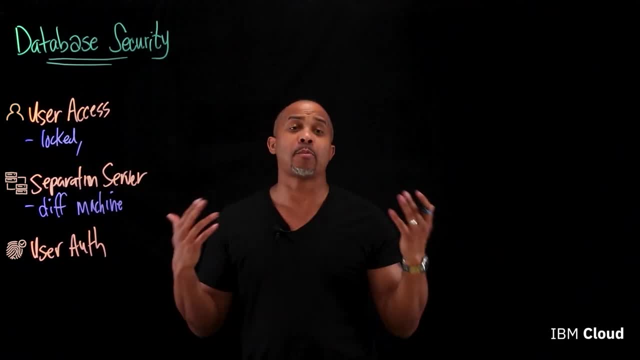 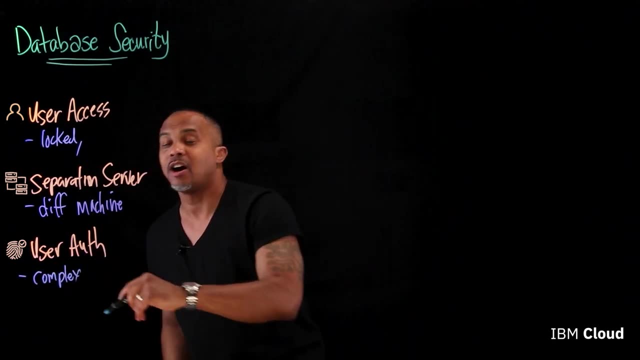 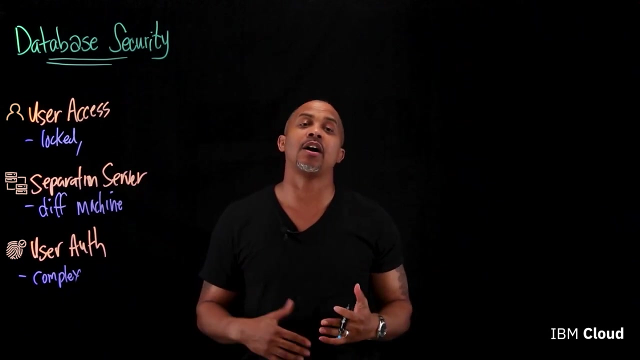 it said that almost 80% of compromises are from password selection. So make sure you get complex passwords. Avoid the usual standard passwords that are there: 1,, 2,, 3,, 4, 5.. Really figure out some complexity of characters, numbers and special characters. 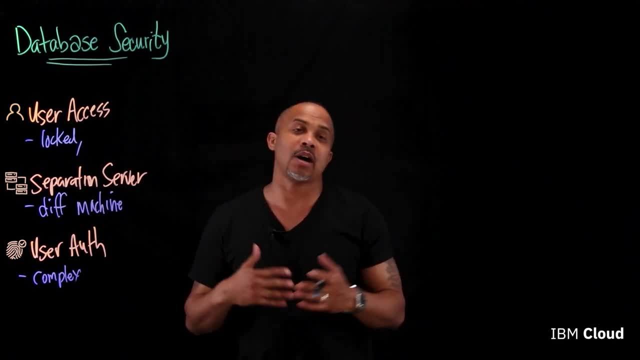 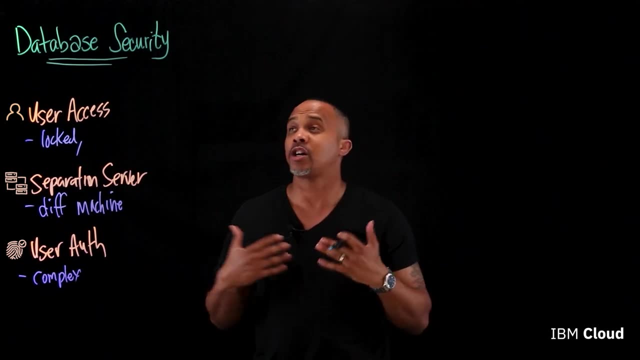 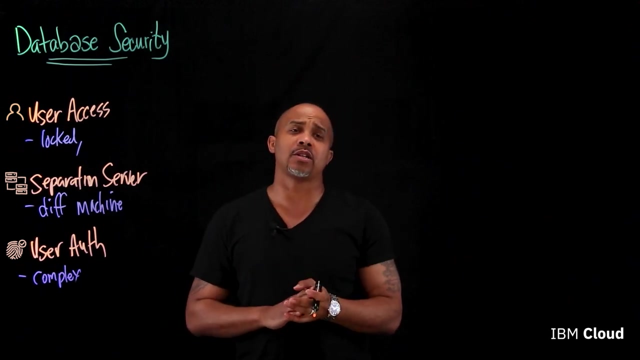 And maybe increase the limit out to at least be up to more than 10 characters. Really just figure out your complexity there, what your policy should be in that use case And then also if you do have sensitive information, like we were just discussing. 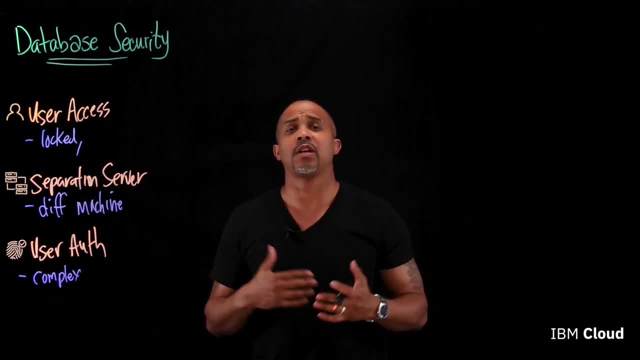 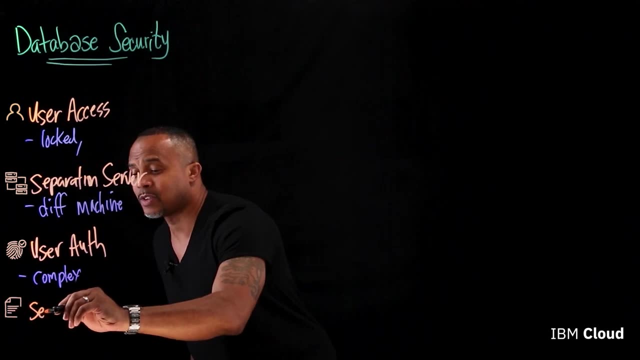 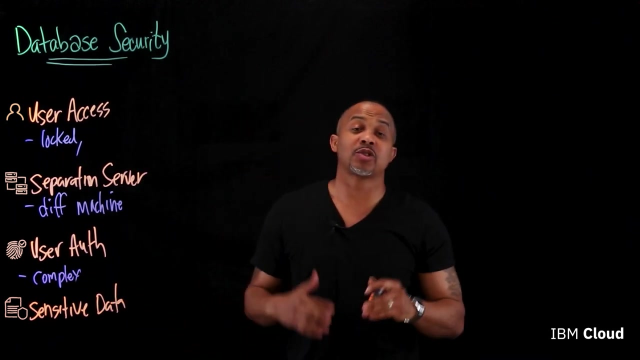 figure out what the context of the application is. If it is an e-commerce application, we do realize that at some point you're going to have sensitive data And in those scenarios you want to make sure you probably consider having some encryption at rest. 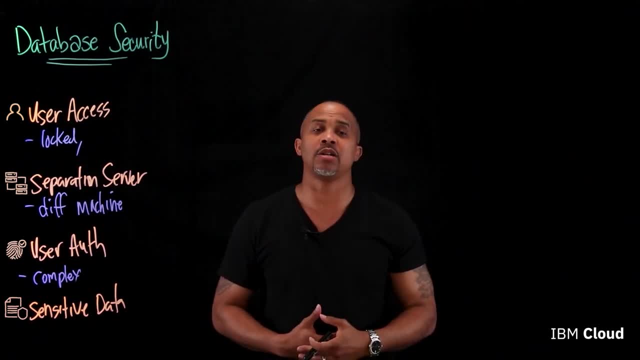 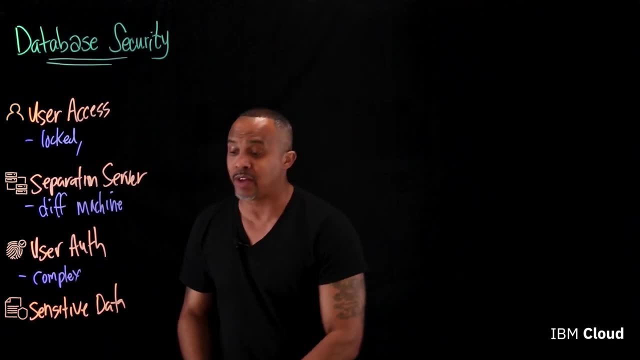 If data must sit, if you must hold credit card information, make sure you actually plan out for how you do your encryption and decryption. This is actually another way that most will actually leverage a third-party provider where you don't really have to store any sensitive information. 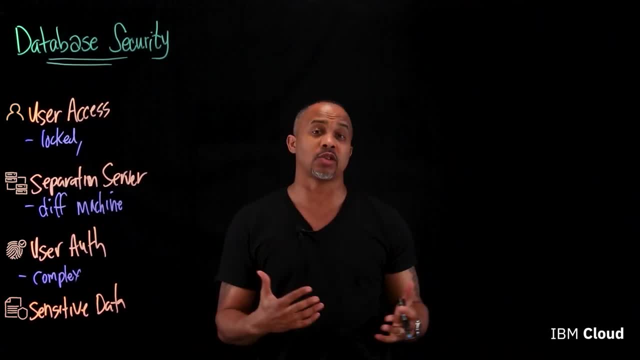 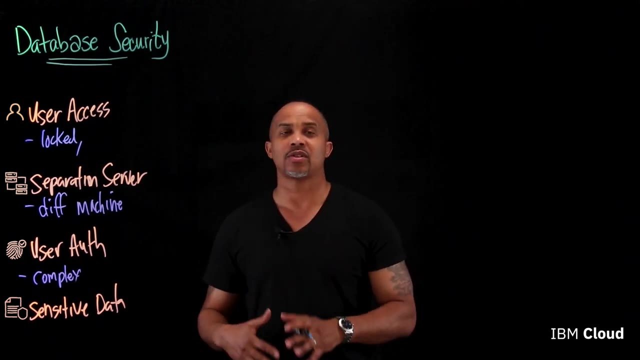 It can list on a third-party service which usually is already set up to be compliant for security. have those in place? So if you're not up to the particular situation of planning for those contingencies, please consider using an outside service which is already set up to use those. 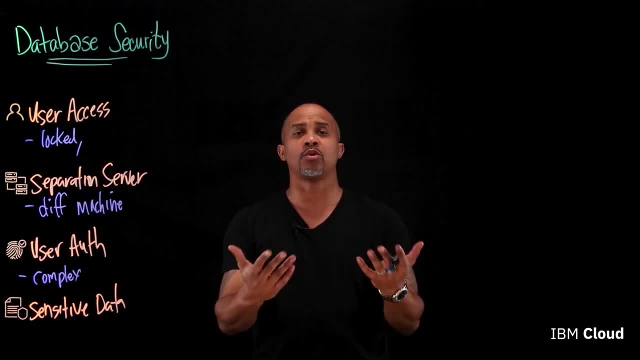 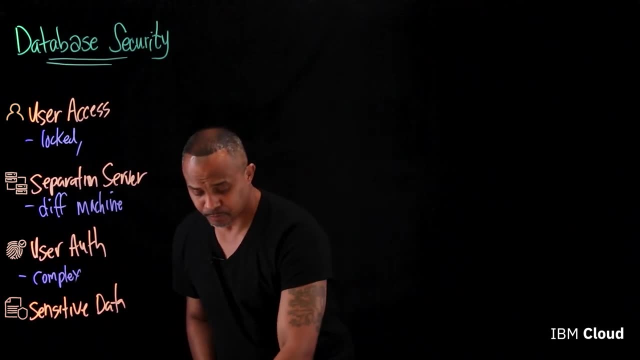 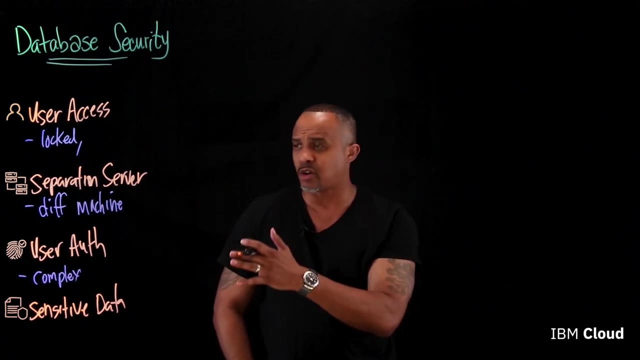 And most of those services will have proper ways that you can pull data in and out on demand as you need, usually normally through REST APIs here. Okay, let's move over to my next four that we'll use. And so we talked about physical access. 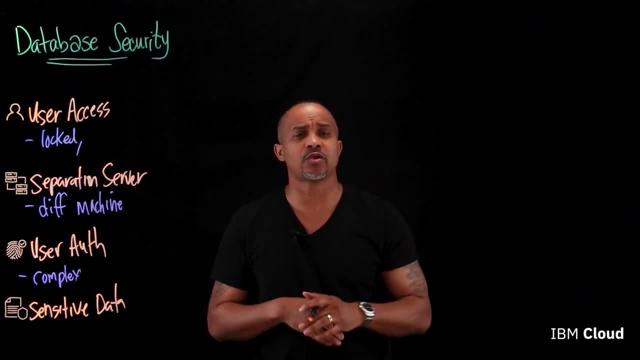 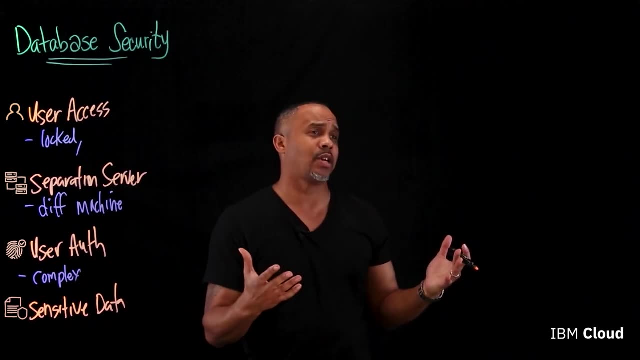 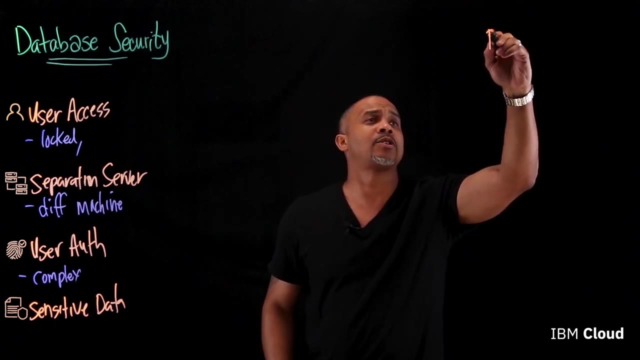 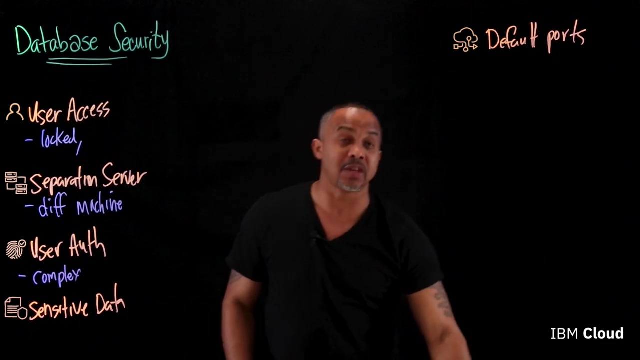 which users have access, keeping separation of those servers, those complex passwords, and making sure we have encryption there, just in case data must sit at REST. Let's talk about the first. next thing is most database servers. they have published default ports, So you want to make sure that you naturally 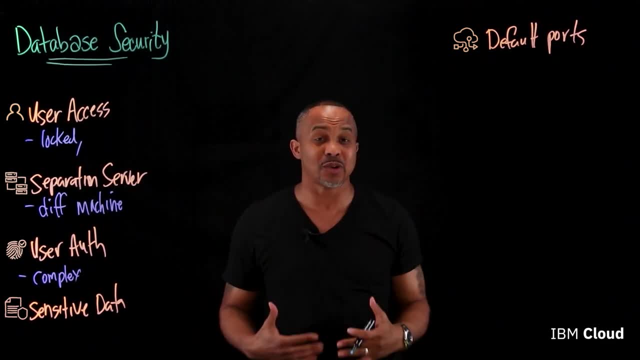 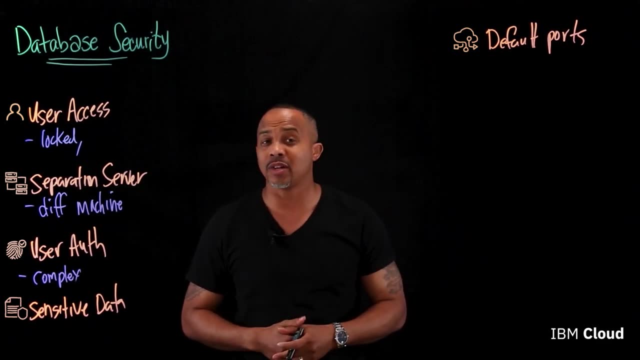 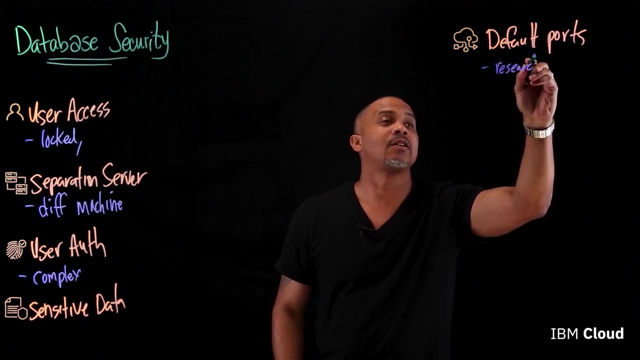 these are things that most of these databases can be run locally. I can stage them up pretty easily. I know like MySQL is 3306, you have Mongo 27017, these are all common published ports So anyone can research these. Now, in the actual cybersecurity world, 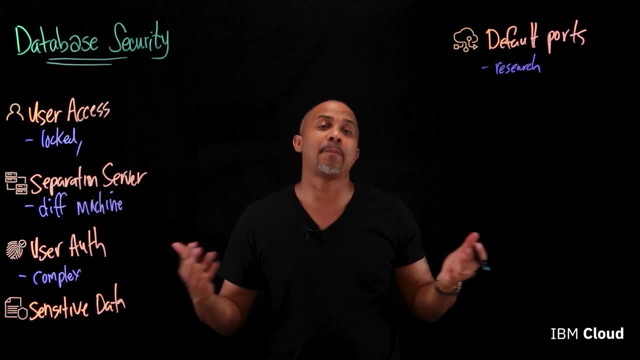 on most OSs, especially Linux. there is a popular utility you can use to run scans on different VMs over the internet, especially if you have a public IP address. So if I do a scan and it comes up that 3306 is active, then it immediately lets me know you're. 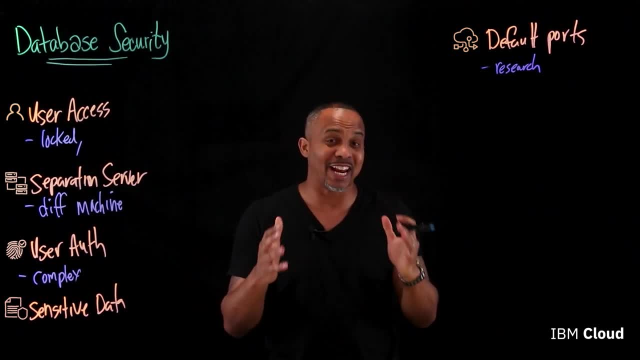 running MySQL database server on that actual server. So you want to kind of really obfuscate these particular details from being so easily used. And if you want to take that concept way beyond databases, we can also use that for just normal SSH access. You know the standard port. 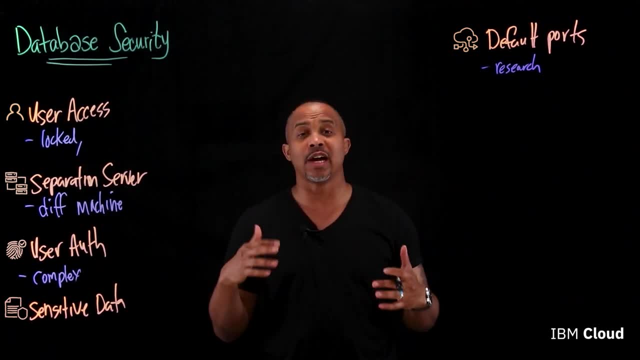 for that is 22.. We can probably run that on something like 2222, you know something that's non-standard. So any of those services that you want to go live with, just do your research and understand, have a strategy in place on ways that you can use that And if you're using that across. 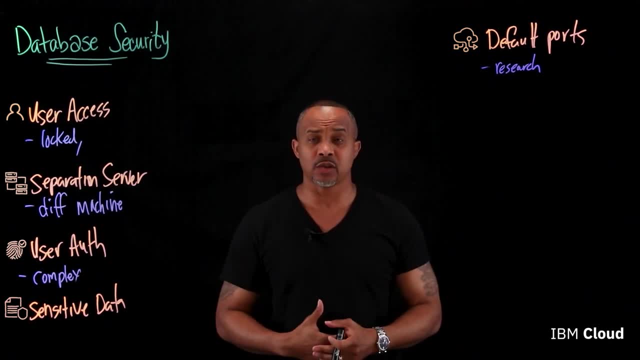 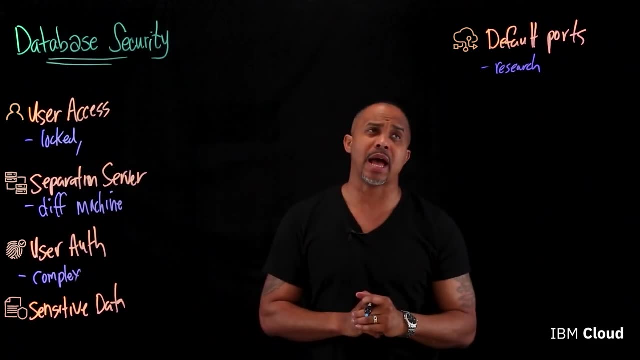 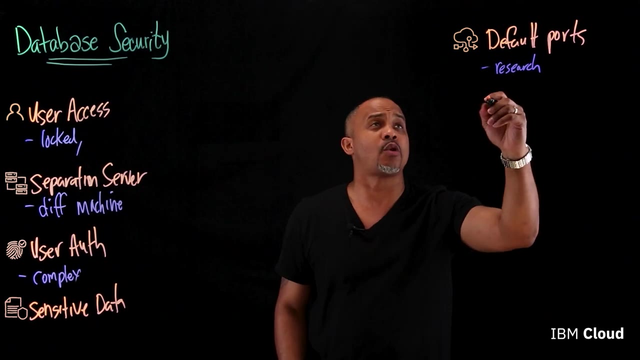 multiple servers. let's say you're managing a farm of these. maybe it'll be a standard port that you choose to run across those, So everyone always knows the pattern that you're going to use. Now, of course, for any of these situations, whether you want to change the port most. 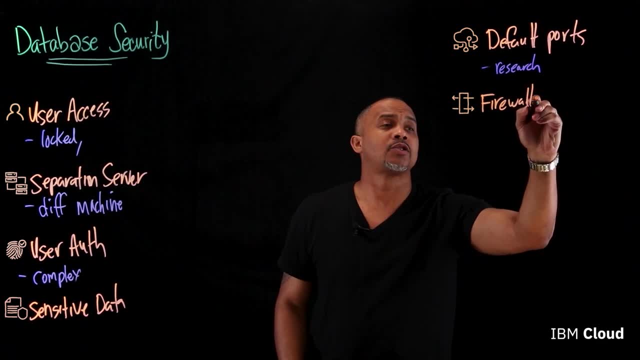 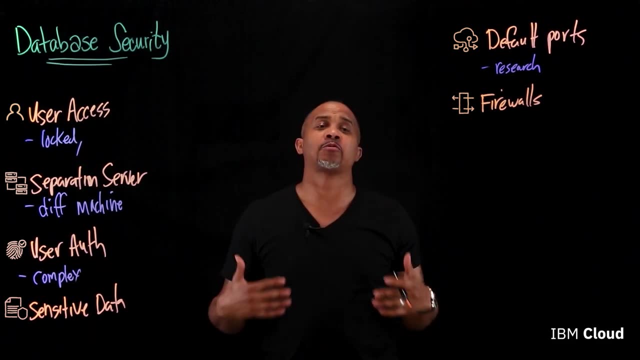 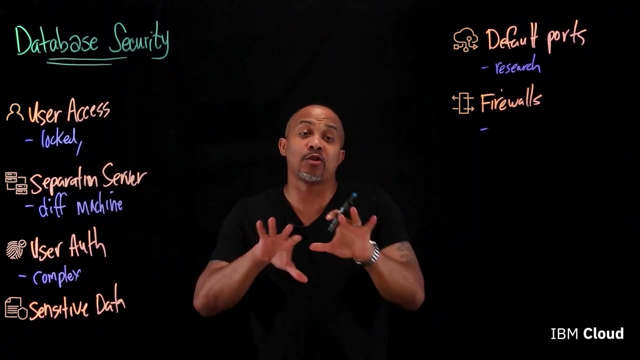 servers. if it's an OS that you're doing, or we'll just talk about OSs now. So you're doing a Linux OS, they're going to have particular firewalls that are available here And with that you want to, probably, if the goal is that you have those. 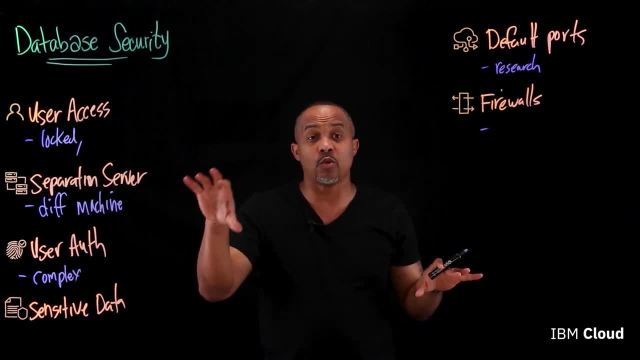 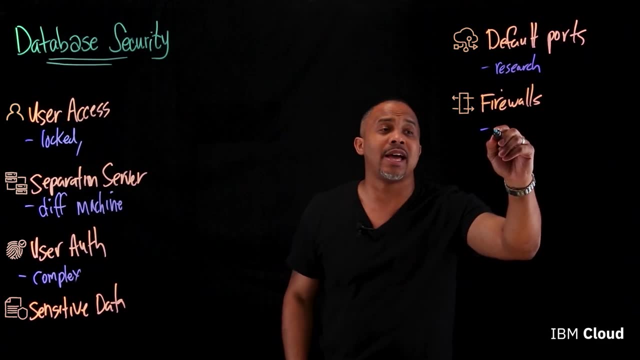 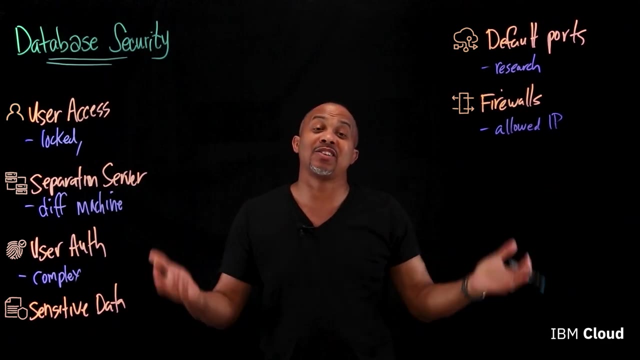 separate servers and only there's only one machine that will be available to communicate with that server. go ahead and put that server in as a allowed IP address- Okay, Rather than standard. by default, most services may come up and say access from anywhere, But if you only know. 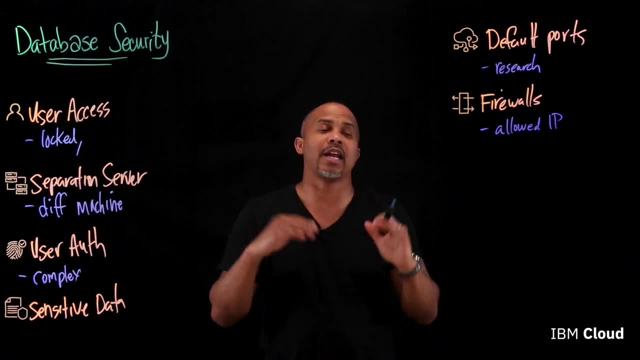 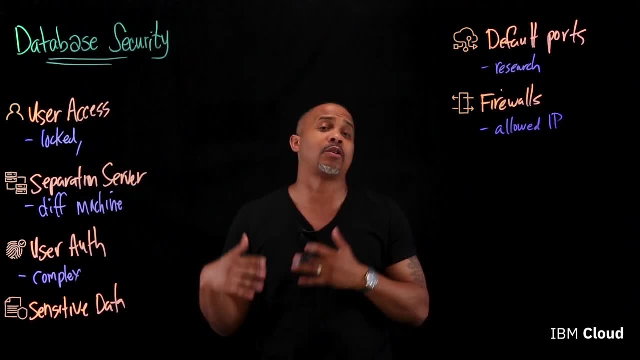 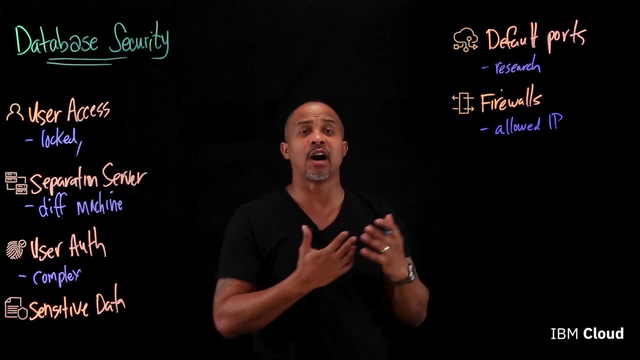 You can also do the same thing. I know, if I subscribe to a service like on IBM Cloud, if I know that my remote server is only coming from one IP address, that should be what you do: Only allow those to come in, All right. And maybe if you're working from your own headquarters or 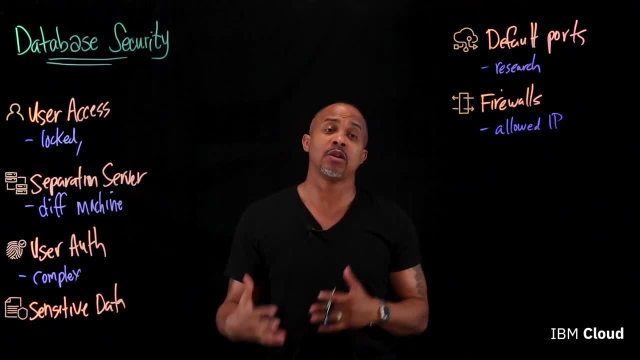 place that you do development, add in those IPs as well to come. Now I know what you're probably thinking. Hey Jamil, it is kind of easy to change your IP address, But for those individuals you really must know what you're doing to try and get those IP addresses. So if you're working from 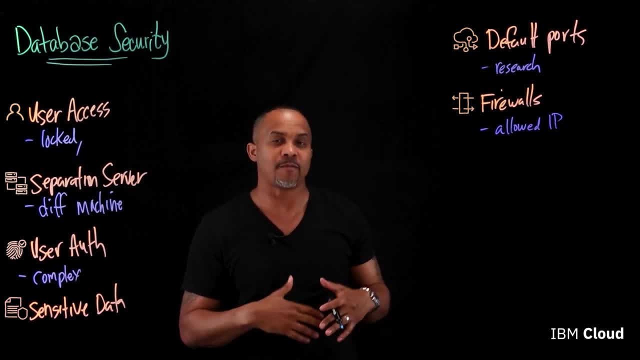 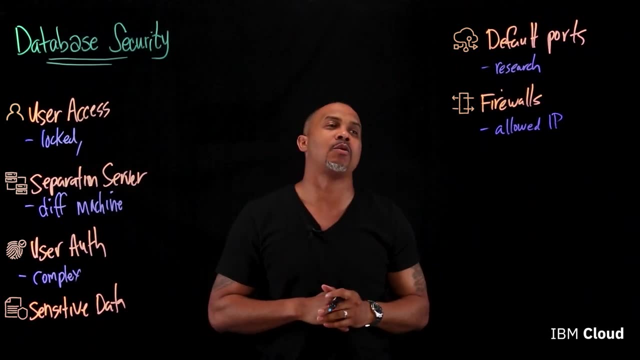 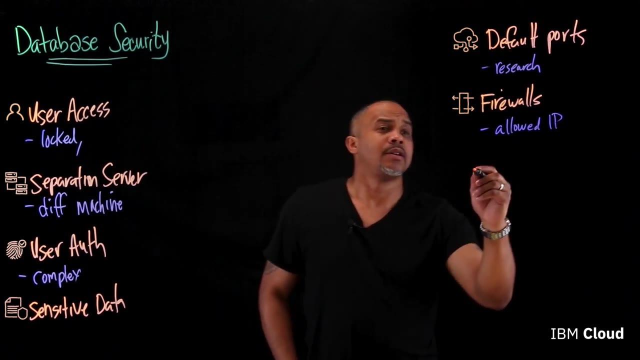 one IP address, try to imitate other IP addresses from what you do. It's not an easy kind of hack to kind of do, But for those these additional methods can really go in place to really compound the effect that you can have here. Next, when you're running your database, you want to make sure you 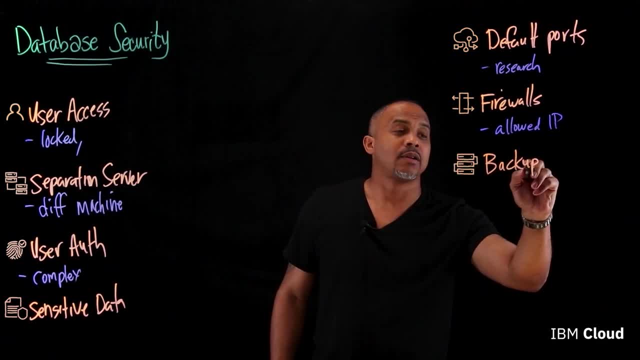 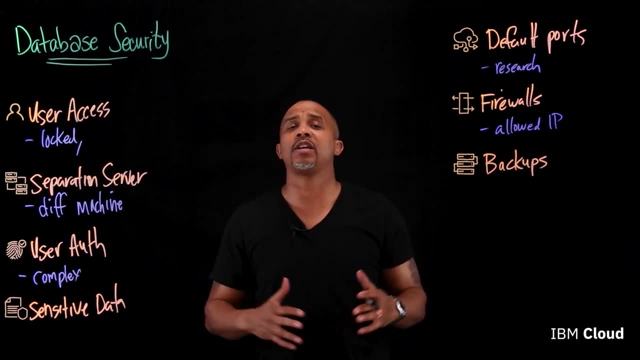 figure out how you're going to do backups, Especially when I started out with LAMP stacks. it's easy to get this whole configuration set up. You can spin up a VM at home or in the cloud for within minutes- maybe less than an hour- And I can. 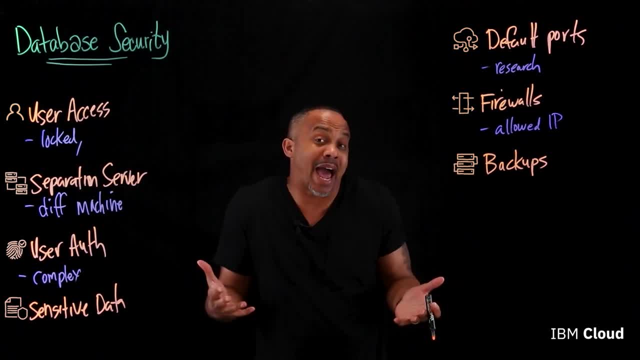 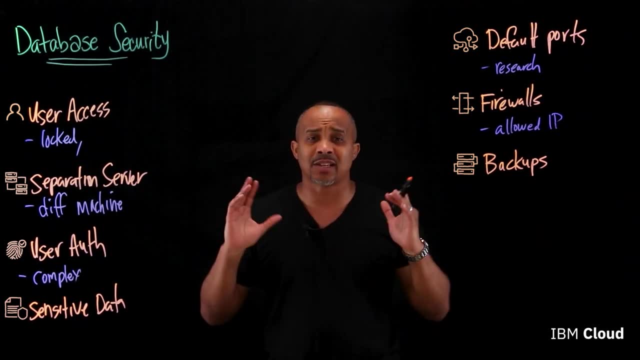 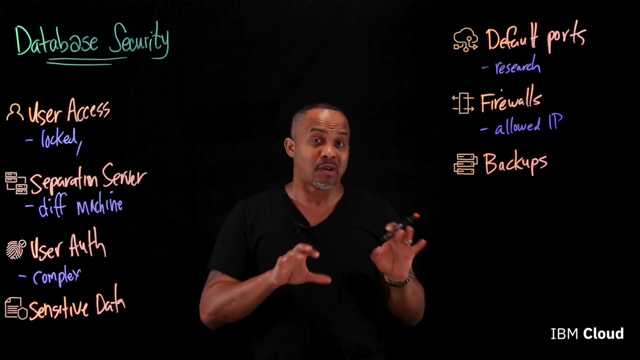 quickly go yum or app, get and install the necessary packages to get Apache, MySQL and your database and your programming language installed. You can be off to the races live, build your site, code it up, be live. But we want to make sure that we actually are able to go through the process of backing up. 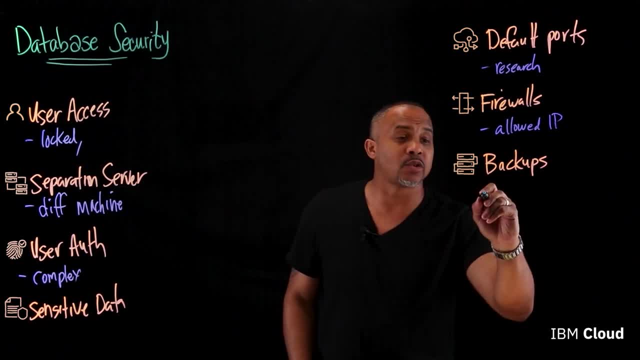 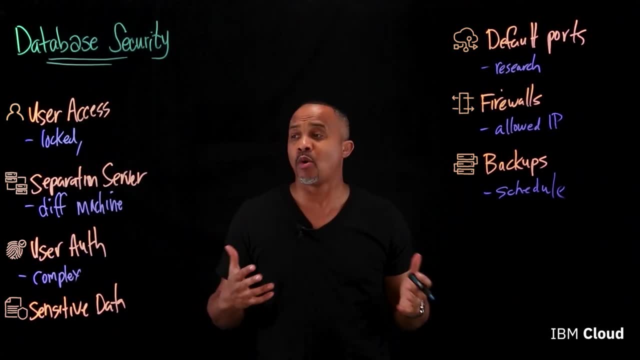 and restoring All right. You want to be able to put this on a website and you want to be able to do it on a regular schedule When you will perform this activity and, most importantly, in the situation that you have separate servers and there is an event of a compromise there. you also want 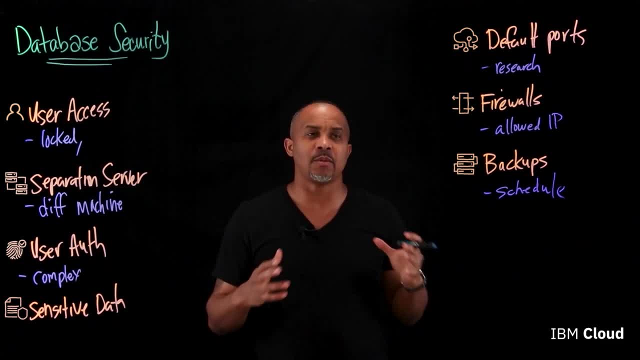 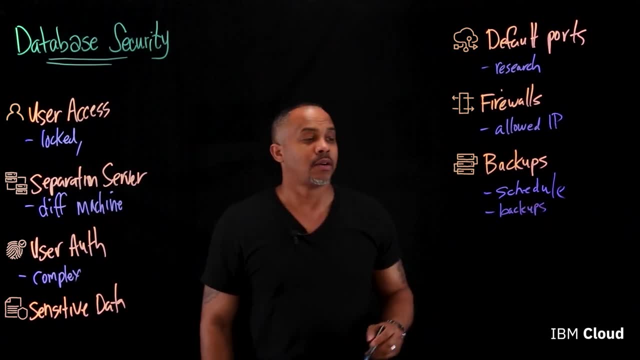 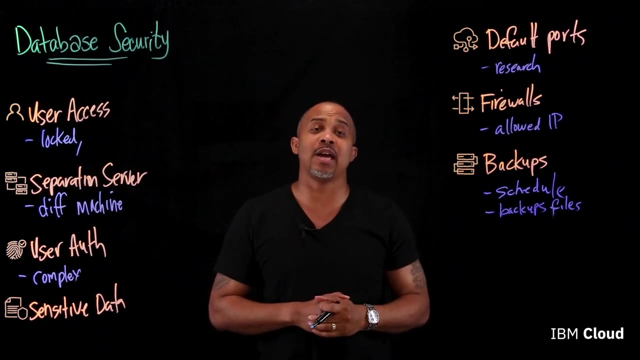 to make sure you have a copy of your data. All right, That is. all is set up, is secure, And wherever you're putting that to the backups, The backup files at that, Make sure that's in a place that is encrypted. All right, So you may- definitely you want to- if you can do that extra step of complexity. 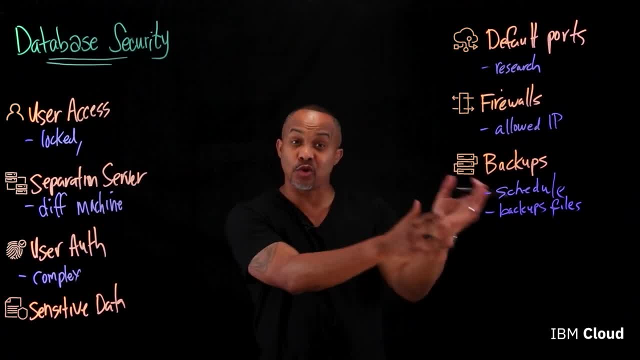 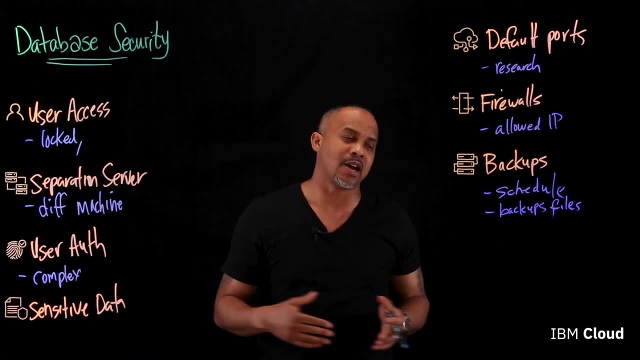 It's not enough that I have a separate database server that I do backups on regularly, Let's say every morning at at midnight, or I mean not midnight, let's say 5 am, 7 am, whatever the actual cadence that you want to run that cron job. But do I really want to keep those on the same? 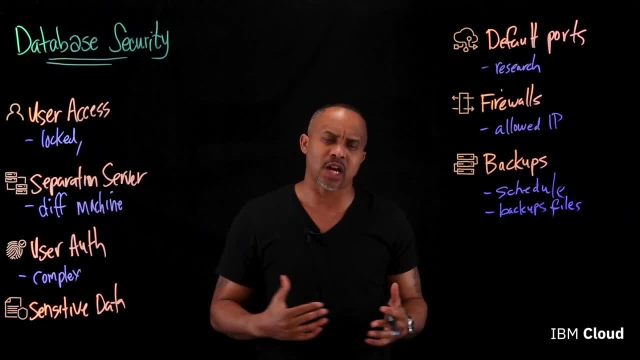 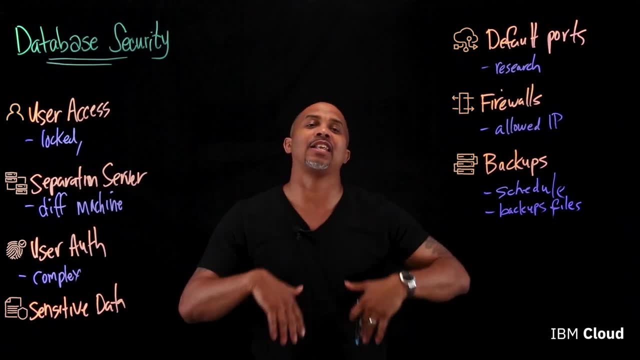 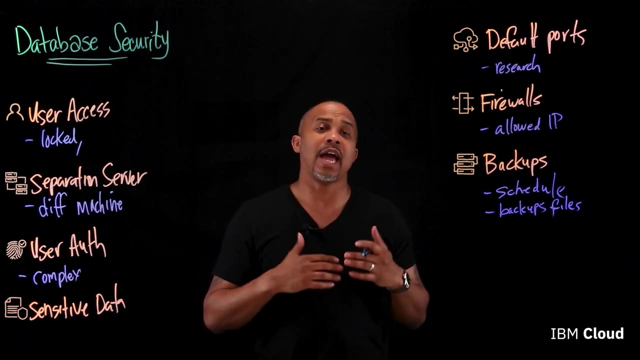 server All right, Because if someone is able to compromise that server, they can easily unzip, back that up or maybe change data and then restore that themselves All right. So definitely make sure you're keeping those backups somewhere that you know is safe and secure And, if possible, if 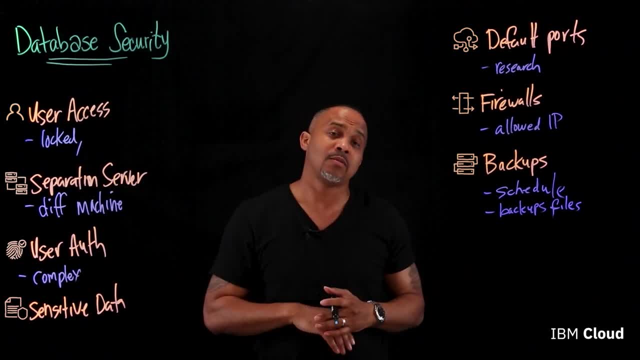 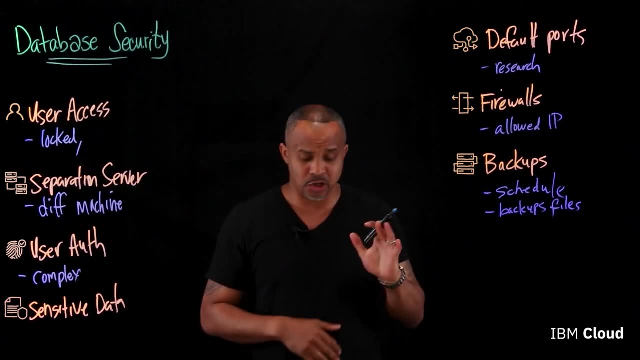 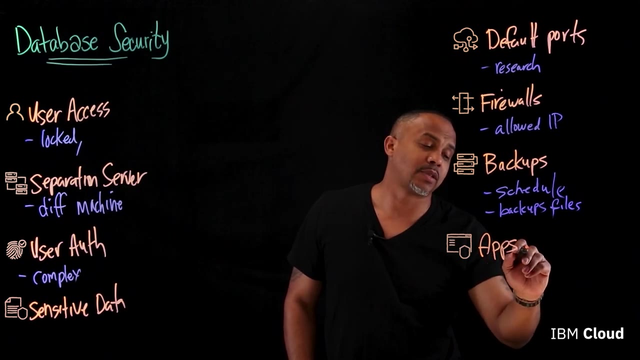 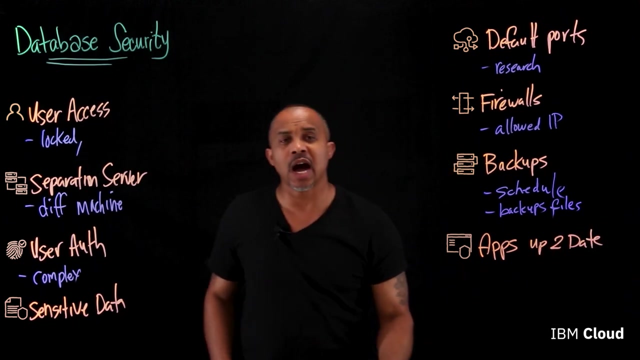 necessary, take extra steps to make sure that those backups can be encrypted in some way, especially if they maintain any sensitive information. And, lastly, I want to say is that we want to make sure we're keeping apps up to date. Now, this is not just for the different database versions. 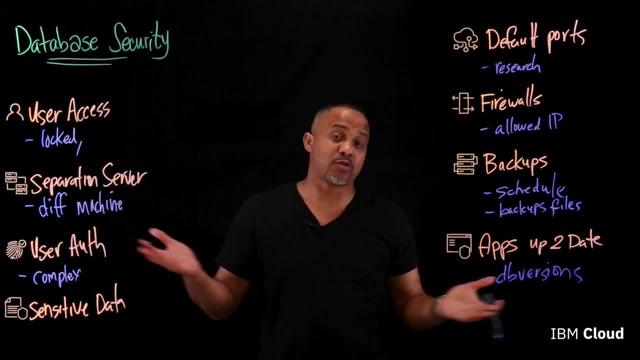 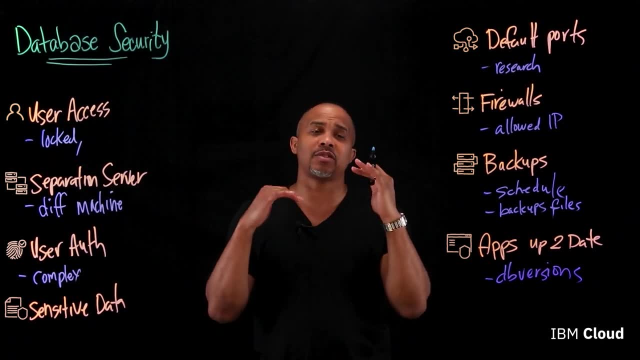 We know that different vendors will allow. like, if you take MySQL, for instance- if I can pick on that for a second- you'll see different versions come out. Make sure you're in depth. You get the announcements for what's changed in different versions as they come out. Make sure that is. 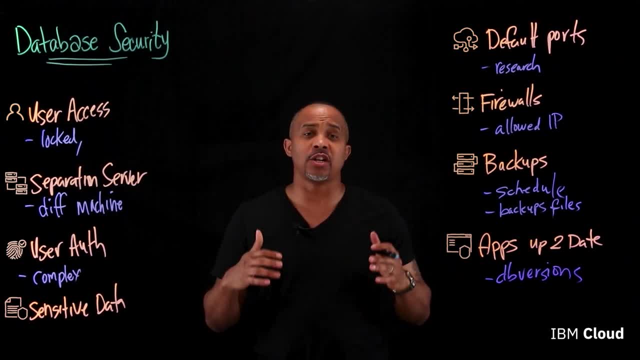 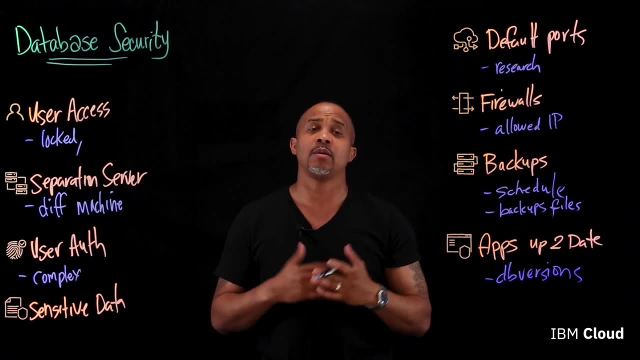 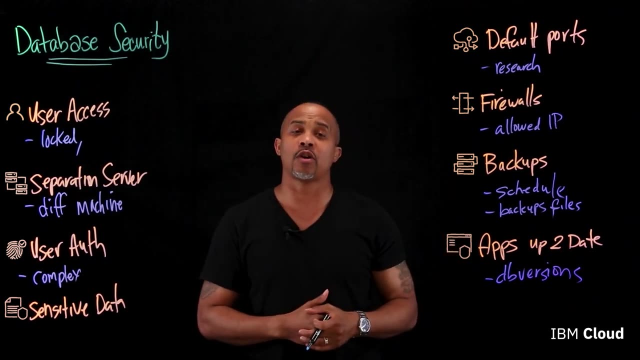 applicable for you. So you want to make sure you have a strategy for how you will upgrade, And that's usually involved. There's really not a concern there if you already plan for your backups. being able to stage a way that you can upgrade your database servers should be as easy as backing up and restoring to a new version with just off the. 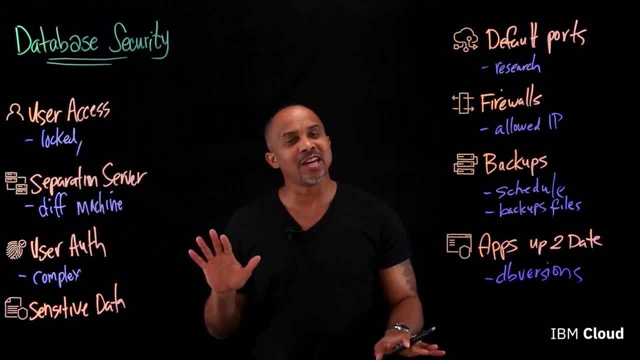 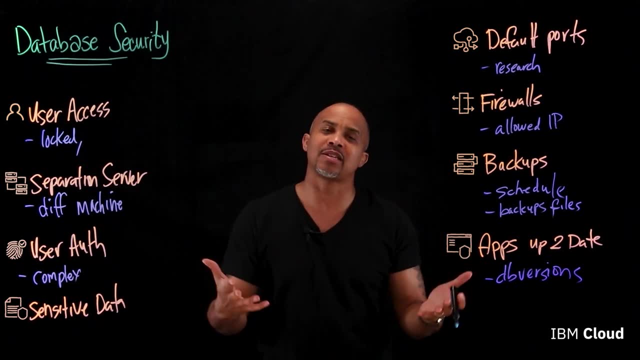 general principle of that. Now, naturally some versions may have changes in underlying infrastructure or the way they're constructed from different versions, So you have to account for that. But usually that does. That information will be actually documented for you to use. 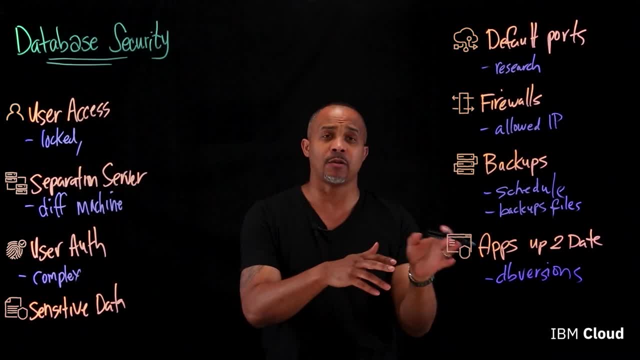 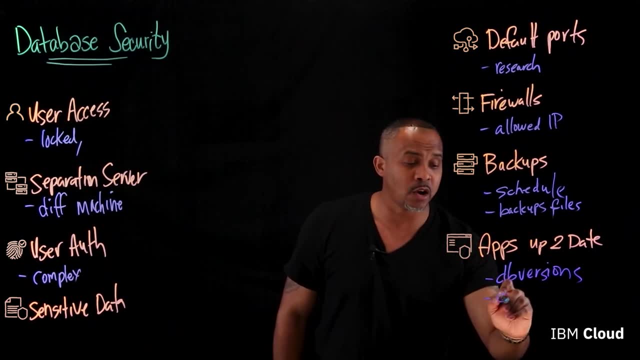 But I want to point out one more thing here on our last note. here It's not just the actual application, MySQL database or the database versions, It's also any code that you write. You want to make sure that those are up to date. 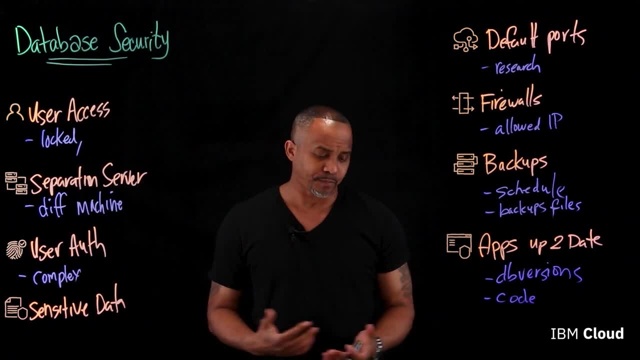 So let's take, for instance- I know it's probably you'll see on the Internet that let's take WordPress, for instance. There are thousands of plugins that are out there. I think a recent survey found that at least more than half of those haven't been updated in years. 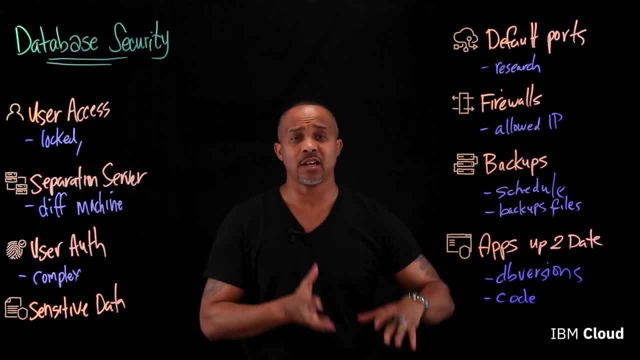 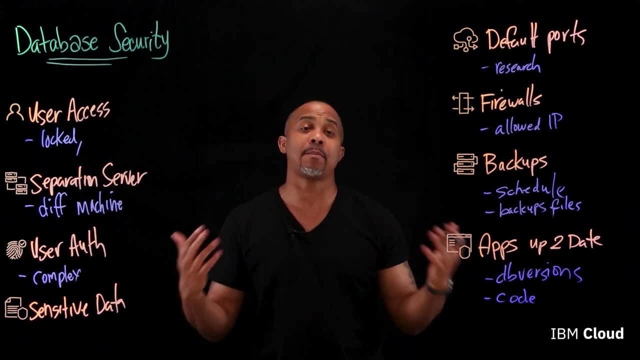 All right. So if I have, I may have my database up to date, secure, with encryption, backed up, have all my walls covered. But let's say I have vulnerabilities in the application that I'm running. Well, if someone can gain access to that application, naturally that will have connections to the database. 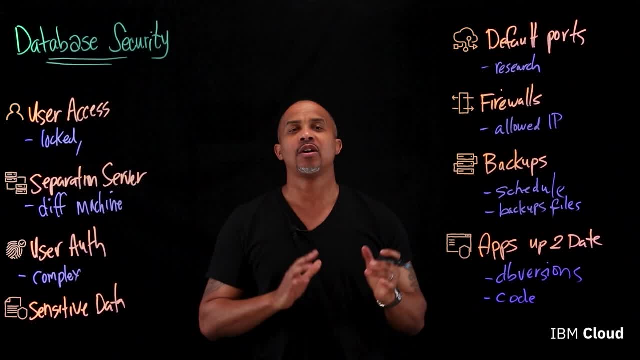 And so it just opens up another door that you don't want to have. So, on top of that, what I'm trying to summarize Here is that, beyond having the actual database at a certain version, make sure that all the code you write is accessing that.